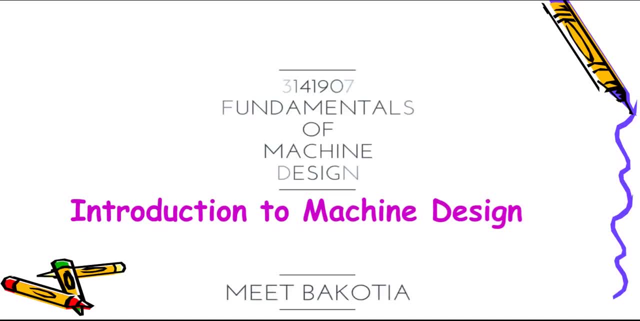 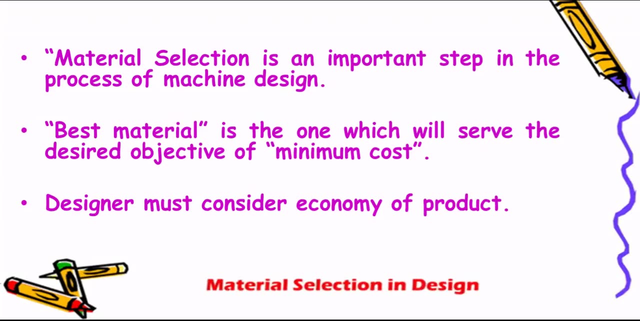 Folks, I welcome you to the chapter number five, introduction to machine design, of 3141907, fundamentals of machine design. Material selection is an important step in the process of machine design. Best material is the one which will serve the desired objective of minimum cost. 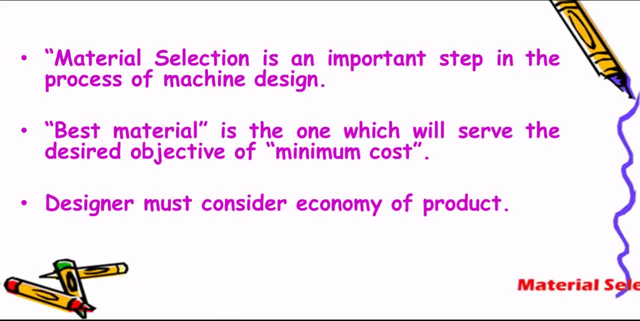 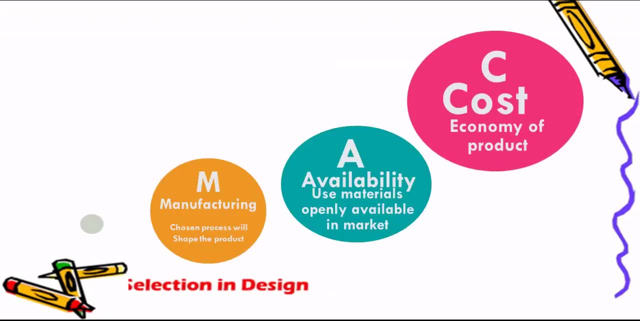 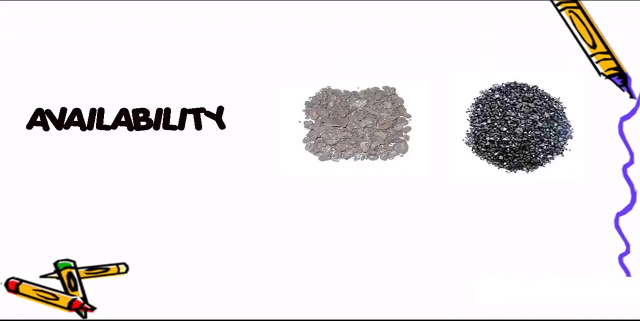 Hence designer must consider economy as one of this important criteria for material selection in design. The four main points that are considered in material selection and design are cost, availability, manufacturing and mechanical properties. Okay, The first is availability. Variety of materials can be used for manufacturing of product. 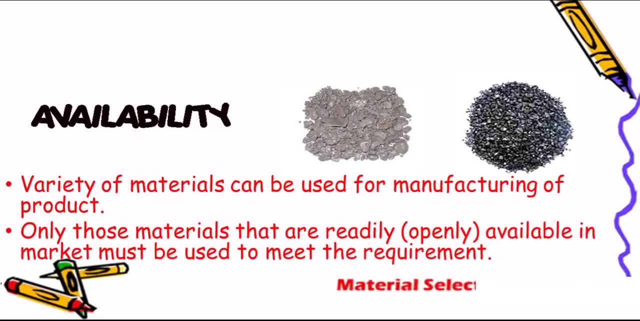 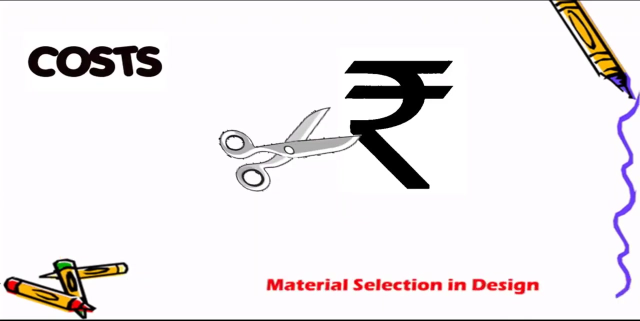 Only those materials that are readily available in market must be used to meet the requirement. Cast iron, aluminum are readily available in the market. Hence those products, materials which are available in the market selected first as compared to those which are not available. Cost is an important time factor for material selection in design. True applications will 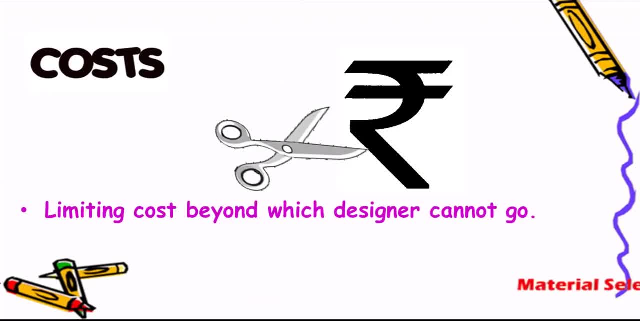 regularly have limits beyond a designer's ability to go beyond. setting Good materials are stuffing material as a number. Price is another very important value in material selection. The designer must select the material which is of optimum cost. For every application there is a limiting cost beyond which 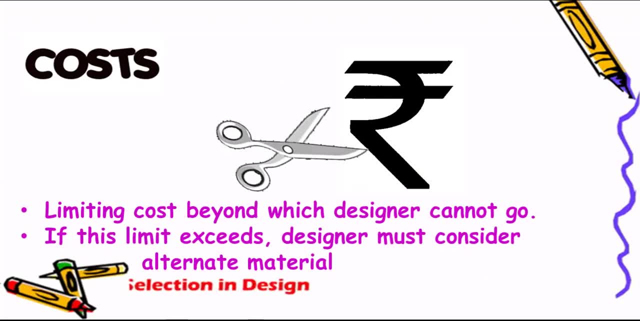 the designer cannot go. When this limit is exceeded, the designer cannot go. Most designers should conduct development of their product imaginatively Later you can discuss this: whether the task of building product plans for any part of their work already done, especially in this designer, has to consider another alternate material. 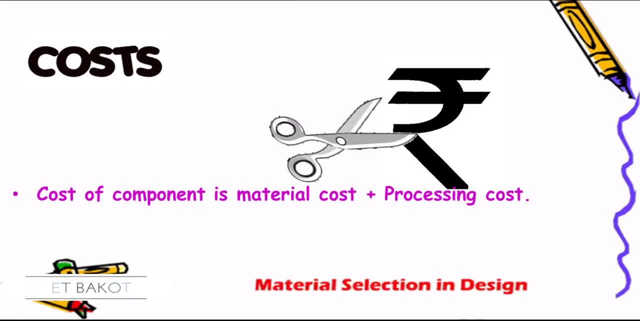 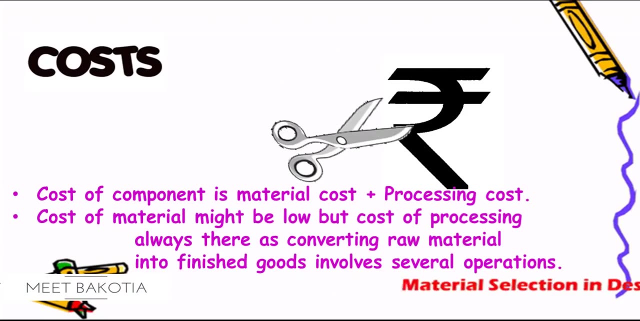 In cost analysis there are two factors, namely cost of material and cost of processing the material into finished goods. It is likely that cost of material might be low, but processing may involve costly operations. Hence there would be some cost of processing for converting raw material into finished 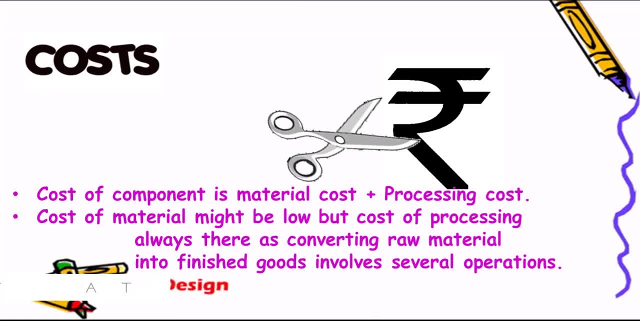 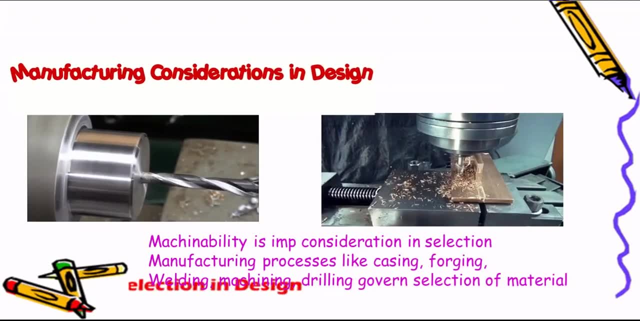 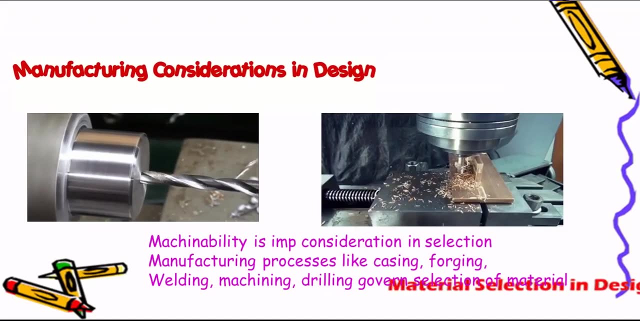 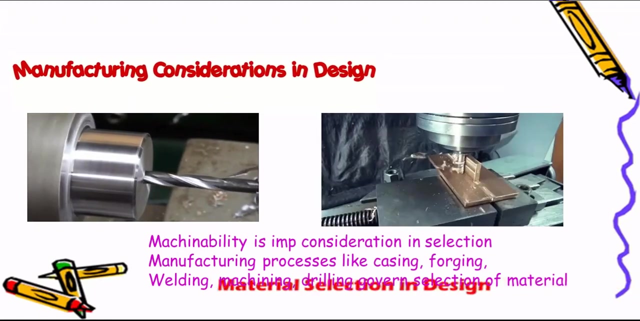 goods. Manufacturing considerations in design. Machinability is important consideration in selection. Manufacturing processes like casting, forging, welding, machining, drilling govern the selection of material. For example, if casting has to be done, then what material to be selected? 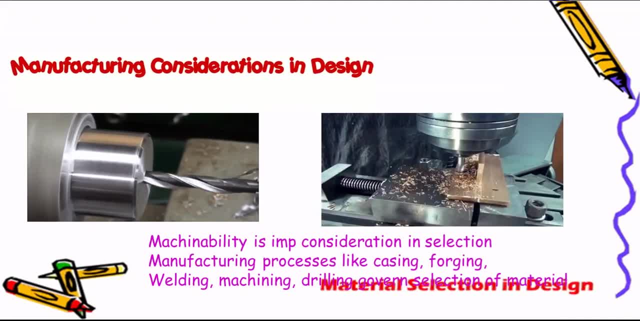 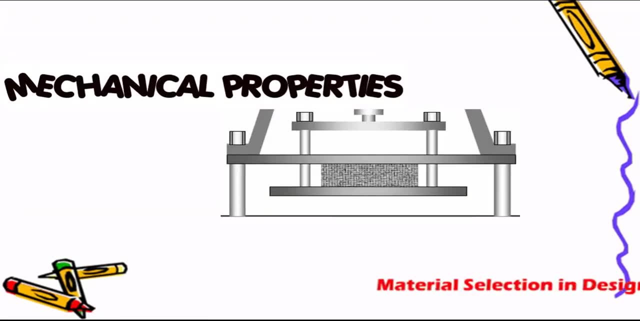 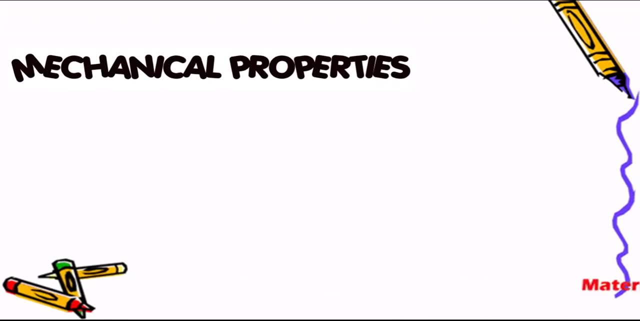 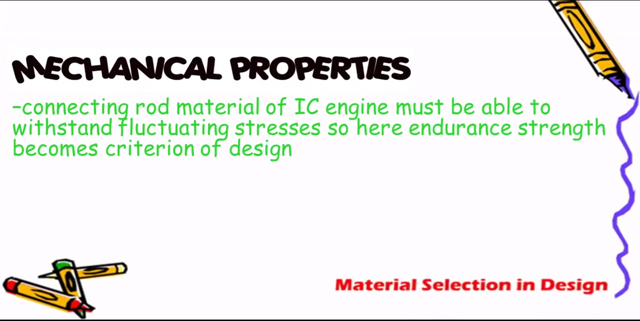 If drilling has to be done, then what material to be selected? Several mechanical properties govern the selection of material. The connecting rod material of IC engine must be able to withstand fluctuating stresses. So here, endurance strength is a mechanical property which becomes criteria of design. 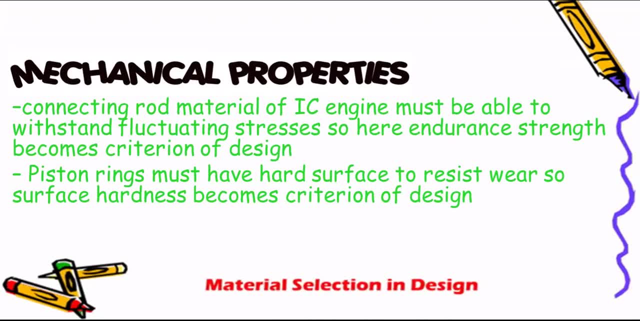 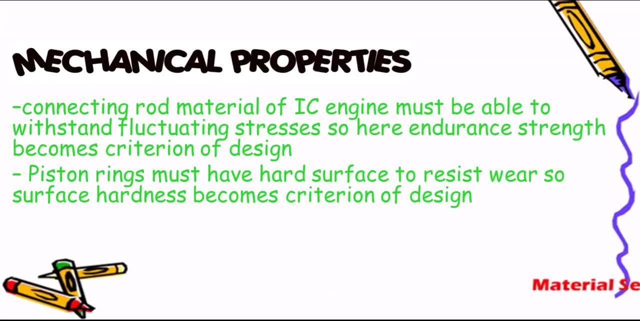 Piston rings must have hard surface to resist wear. So surface hardness is a mechanical property which becomes criteria of design. Thus, there are several mechanical properties on basis of which the material selection should be based. Don't consider hard surface to resist wear. 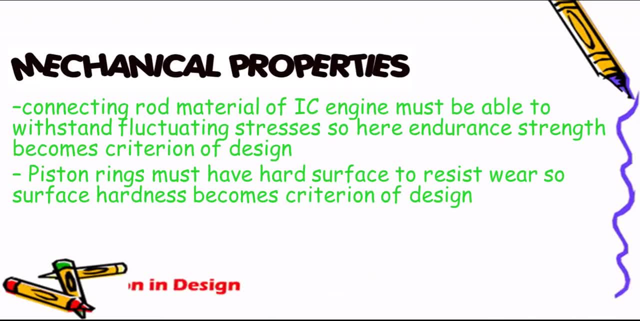 Modulus of elasticity becomes the criteria of design. Hard surface for touching the workpiece, Hard surface for analysing also becomes a keen point forPoster armour- pindch Usd. If toughness is considered, then ISOD impact 4 p test should be большое specific for the 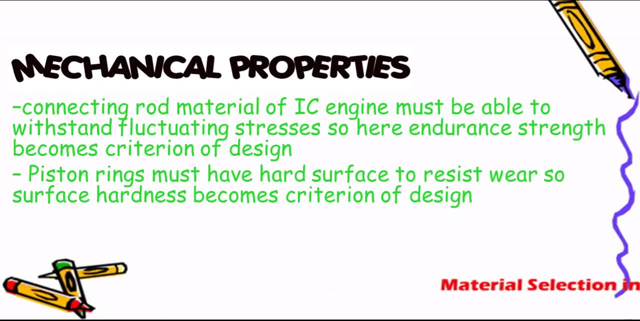 workpiece. hence one special problem in design: Hard surface or patent marks. either bain-marie or neodymium shouldn't be seen and only french or신 atraipass. Microsoft would keep R Rex Te circuit okay. The drawing surface may also require inWhen cast wear is done. 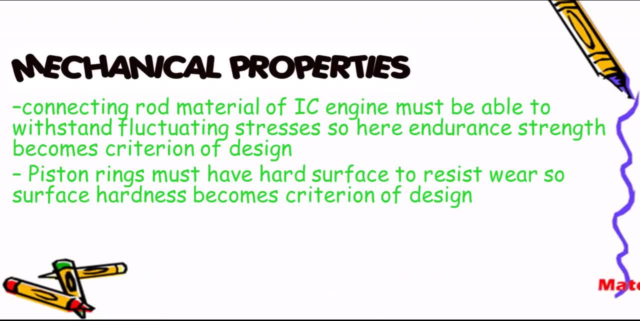 CRPS, steel® or disagre. those components are classified and must be reduced to Мне. the minimum is given up. Worlds ofgers used are the following: be seen if the toughness is within the limit or not, and then the material selection should be done. 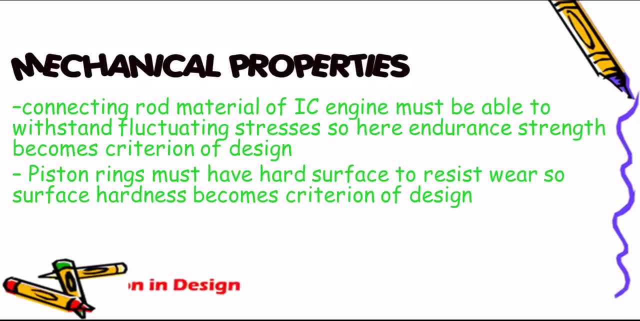 thus four important steps: availability, cost, mechanical properties and manufacturing considerations and design should be considered while material selection in design. thank you,